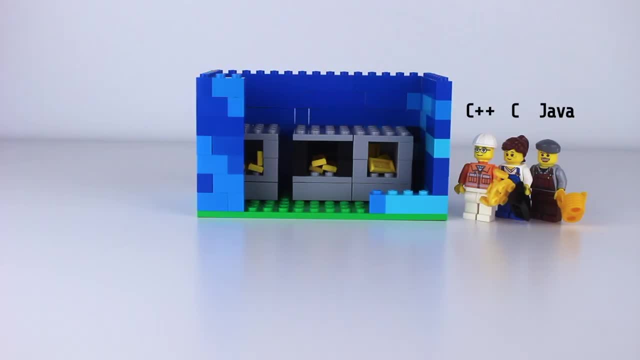 from a database. This warehouse or database stores data from a database. This warehouse or database stores data from a database. This warehouse or database stores data from a database. The warehouse database was built using coding languages like C++ or C or Java. Now imagine regular Lego people. 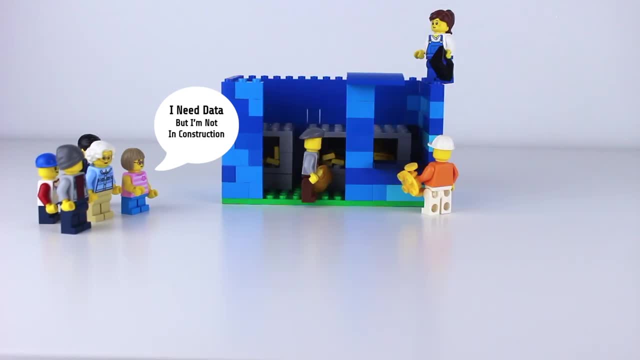 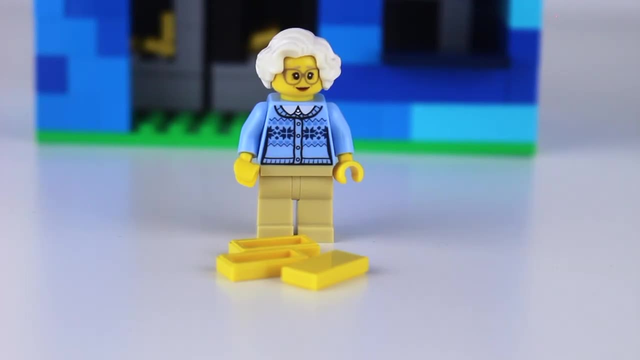 need to access the files. How do they do that? Option one: you could have a storefront built to the warehouse so that customers can ask for files, add files, delete files. But essentially this means you are building something that takes a lot of time, money In the real world. 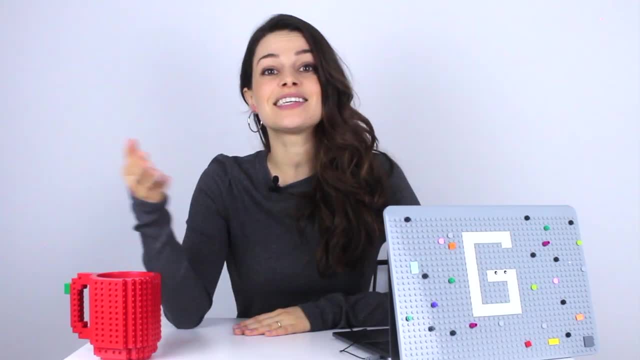 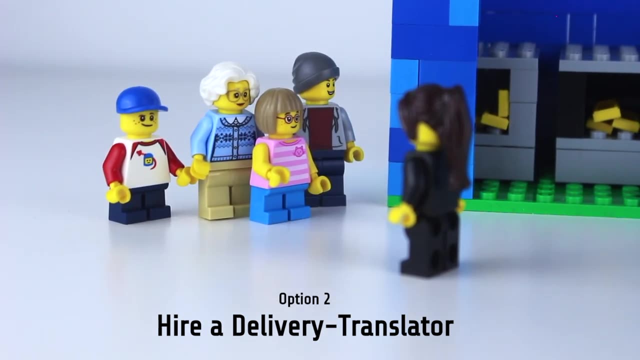 this is the equivalent of building a whole app just to access the files in the database. SQL comes in, which is the second option. SQL comes in, which is the second option. This is like you hiring a specialized delivery translator. Her name is Sally Sequel, She knows. 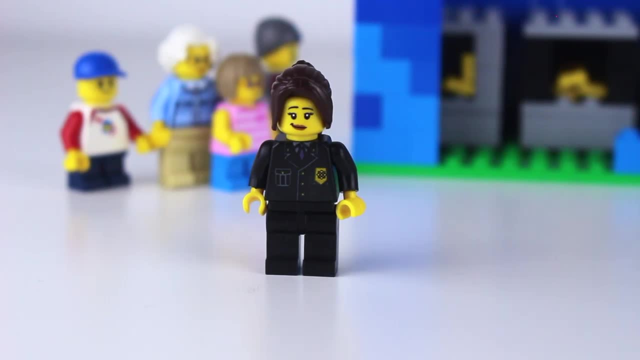 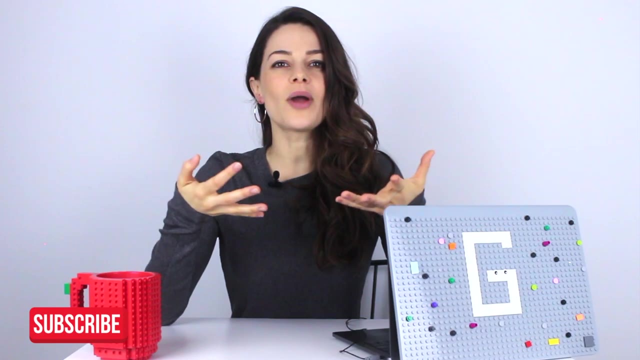 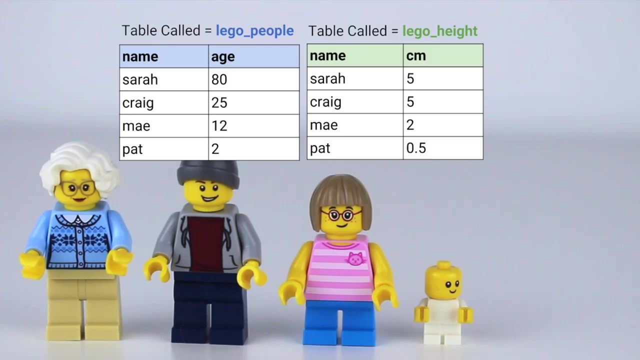 how to talk to the database, and she knows how to speak in the language of SQL. So if you learn to speak SQL, then you can ask her to get files for you. Okay, so how do you speak Sally's SQL language? Here are the requests you could make If you're a Lego mayor. you want to know the 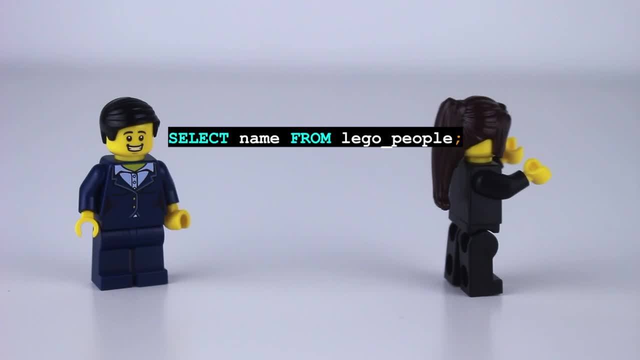 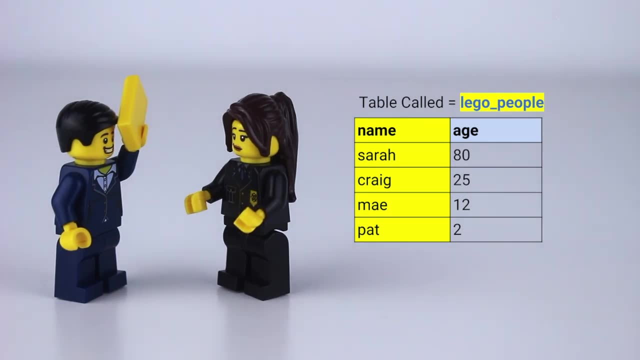 name of your citizens. you'll ask Sally SQL: select name from Lego people- The request to select name that column from Lego people, which is the name of the table. Or if you're a Lego doctor and want to know the name of citizens that are higher than three centimeters, you would 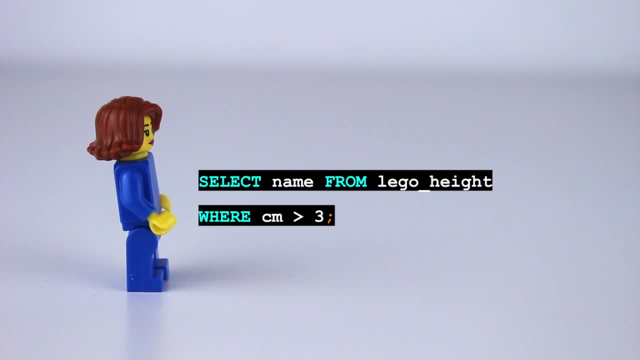 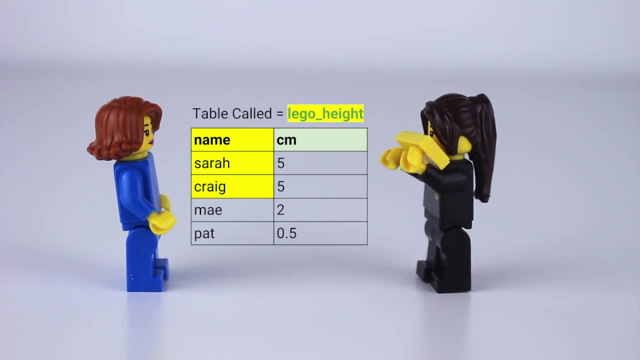 ask Sally SQL: select name from Lego height where a centimeter is greater than three. She returned to Lego people- Sarah and Craig- because their centimeters is greater than three and she pulled from the name column within the table called Lego height. 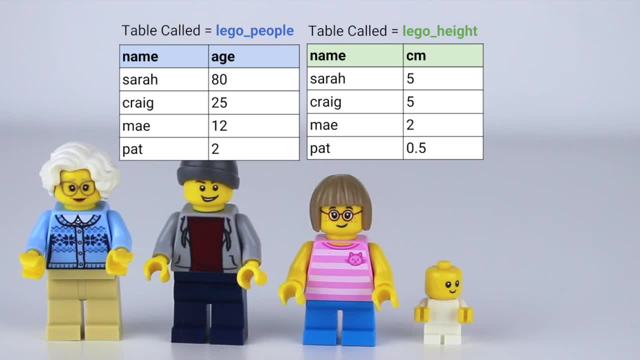 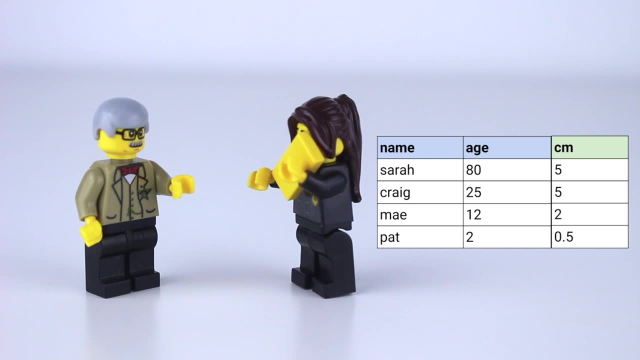 Or if you're a statistician and you want to know both the height and age combination of citizens, data is stored in two separate tables. Here's what you'd say to Sally SQL. Not all tables are found together. Sally joined the two tables because what both two tables had 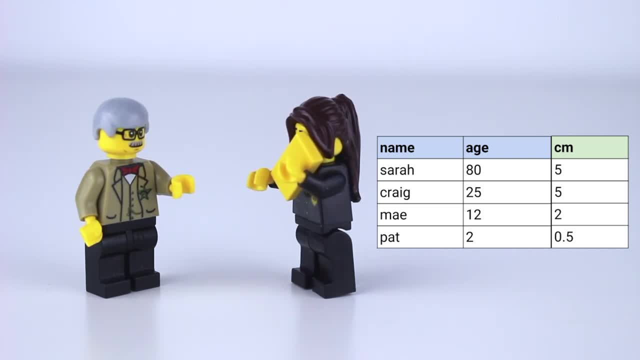 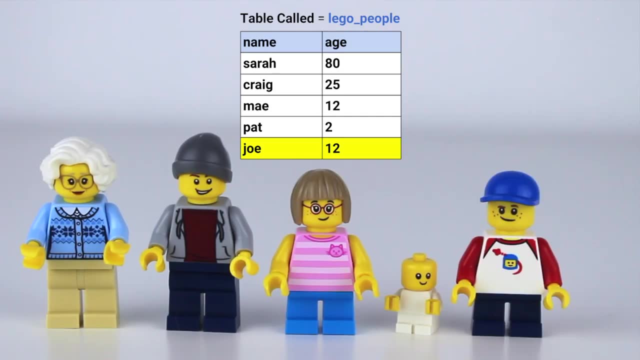 in common a names column. She was able to join the two matching by the names in each table. But you can also do other things. You can add data, If you want to add Joe, who's age 12.. Or you can update data: make Joe 13..